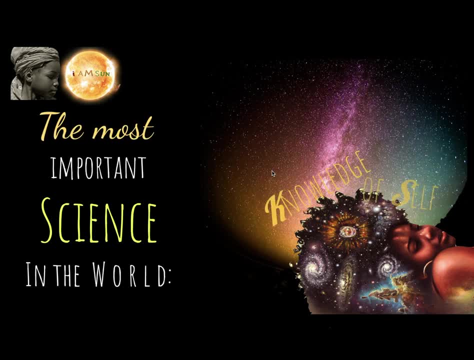 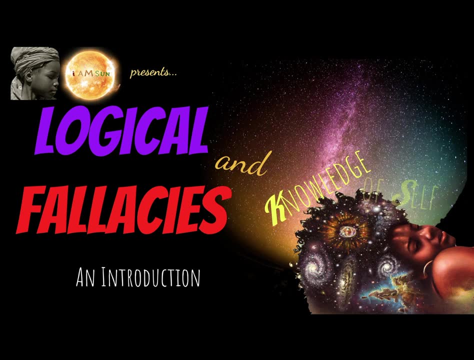 Okay, now we know, the most important science to pay attention to is knowledge of self, Our own set of patterns and what they tell us about ourselves, And we're up on logical fallacies. If you're not, click on the link to the series below and then come on back here, Now that we understand reason. 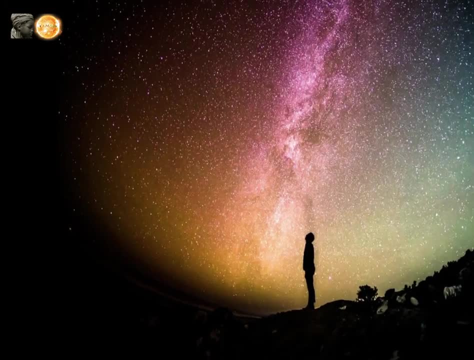 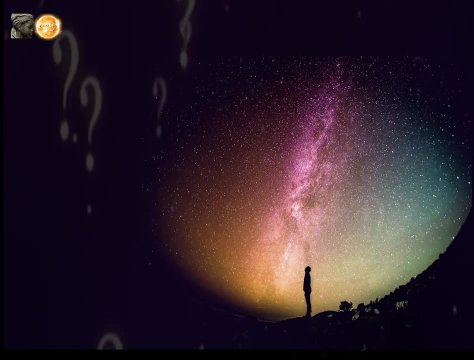 and patterns and the great purpose of knowledge. what about that larger universe around us, the one we're a part of? What are its patterns and what can it tell me about myself? Hmm, what a beautiful question. Have you ever taken a moment to just observe? 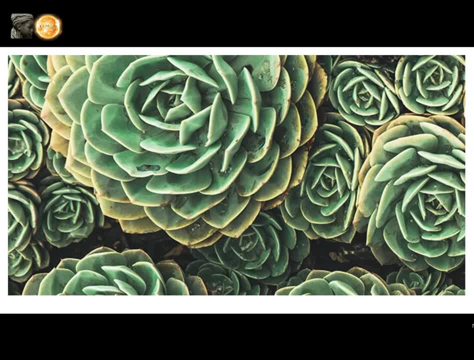 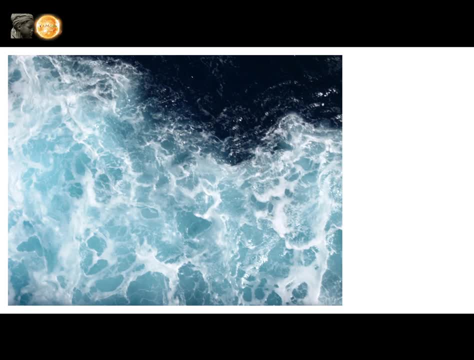 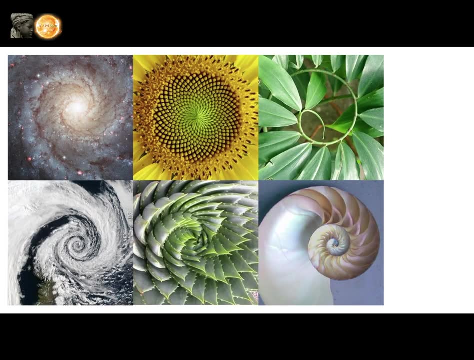 nature, You might start to pick up on something. Let's look From succulents and vegetables to trees and forests, to lightning and waves of all kinds, to canyons and that curious spiral that keeps showing up in so many places. nature is filled with repeating patterns, inside of patterns. 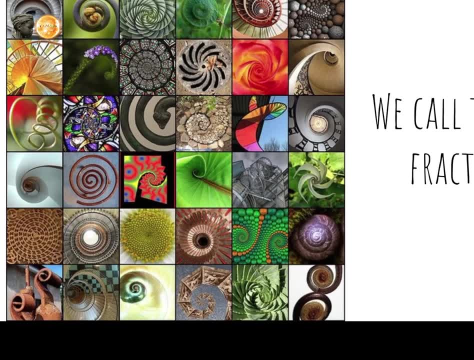 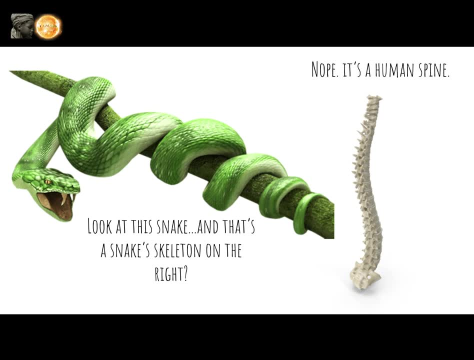 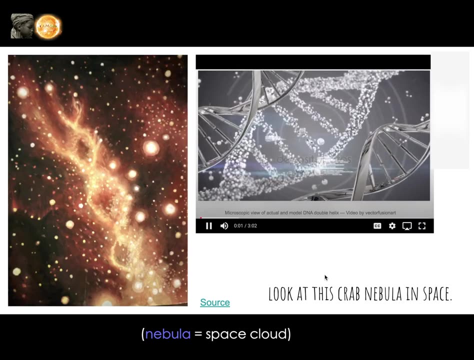 We call them Fractals. Can you say fractals Like look at this snake over here, wrapped up along this branch And that to the right, That's a snake, skeleton right? Nope, It's a human spine. Look at these human eyes and look at these stellar nebulae. Look at this. 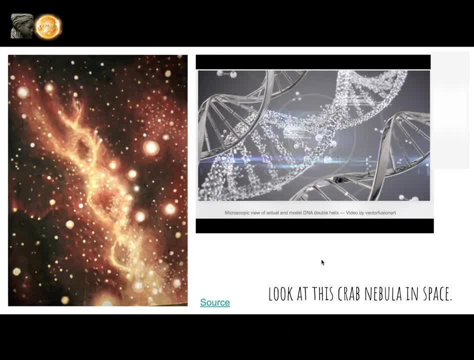 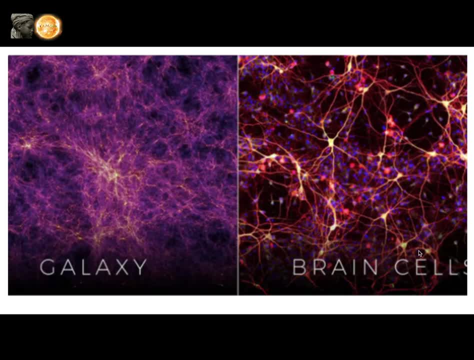 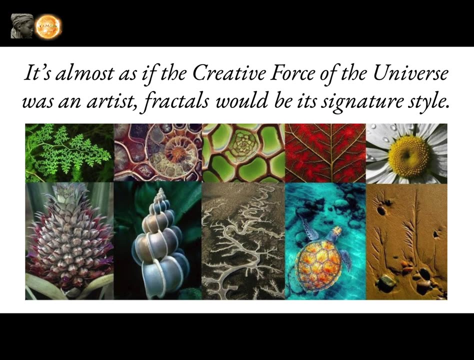 crab nebulae in space. Now look at the DNA in our cells. See a similarity. What about this leaf and a human hand? Even our brain cells look like galaxies from far, far away. It's almost as if the creative force of the universe was an. 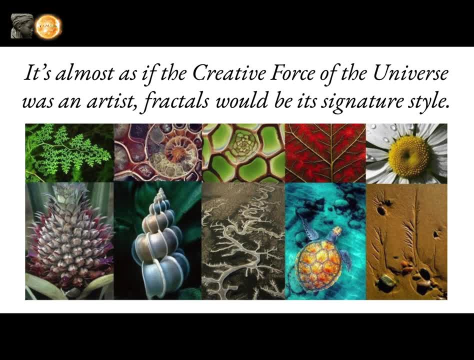 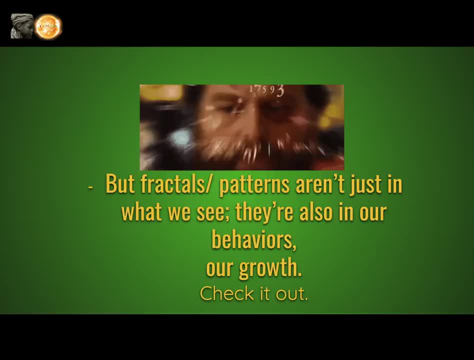 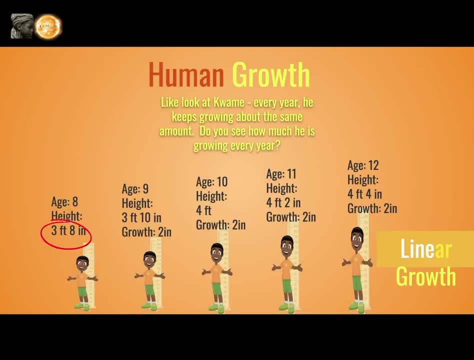 artist, Fractals would be its signature style. just like Picasso has a recognizable style and Kehinde Wiley has a recognizable style, so does the universe. But fractals or patterns aren't just in what we see. they're also in our behaviors, our growth, Like. look at Kwame. Every year he keeps growing about the. 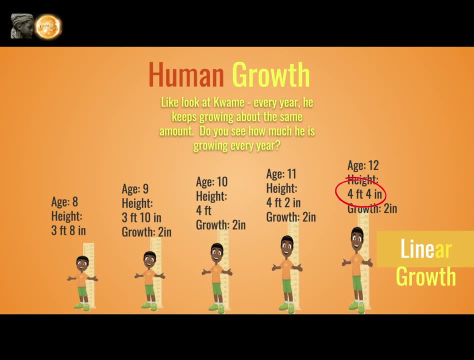 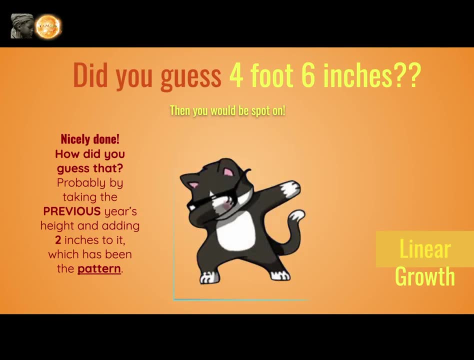 same amount. Do you see how much he's growing every year? Did you say two insects inches? Very good, Can you tell how much he might grow to by the time he's 13?? Did you say four foot six? You are correct. Patterns help us predict. By noticing a growth pattern, we can predict where.